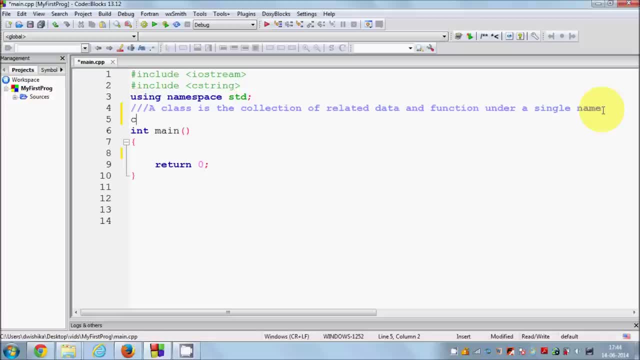 declare a class in C++ using the name class itself and then you give the name to your class. Generally, it's a good practice to start your class name with a capital letter. So, for example, I want to make a class called book, So I will write this class as books. 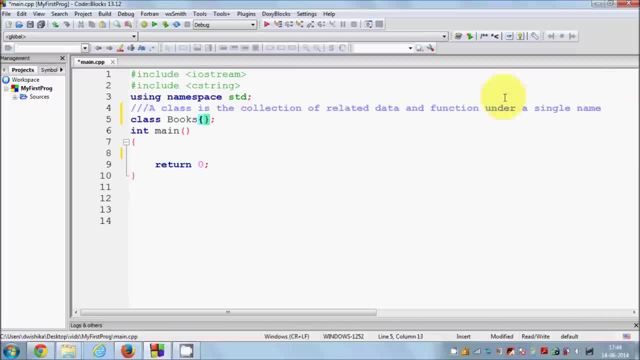 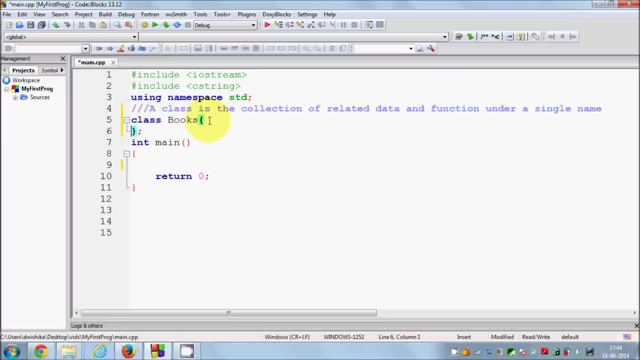 and then you give these parenthesis and this semicolon. So this is a basic definition of class, and inside your class you can declare different variables or different functions. Now there is a word called access specifier. Now, for example, if you want to use variables, 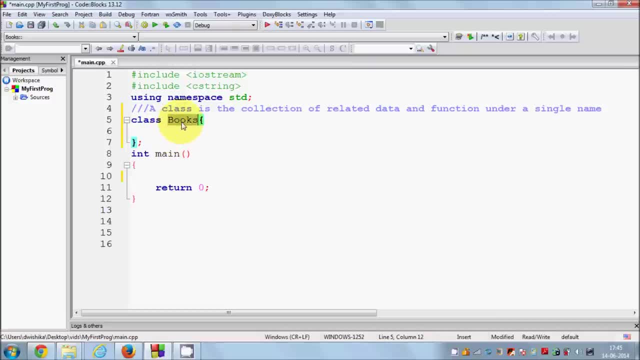 or function which you declare inside this class in your main program. So the functions in book class. you want to use it in your main program. You use public access specifier Or otherwise. if you don't want to use your function inside your class and you just want. 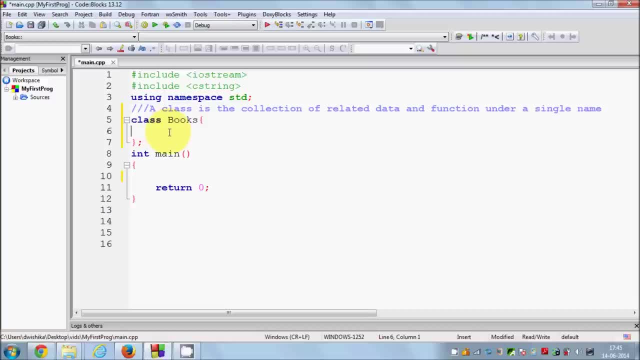 to use your function inside your class, inside your class itself, then you need to use private access specifier. But this I will explain you later. Right now we are going to use a public access specifier, So you can declare this public access specifier like this, Just. 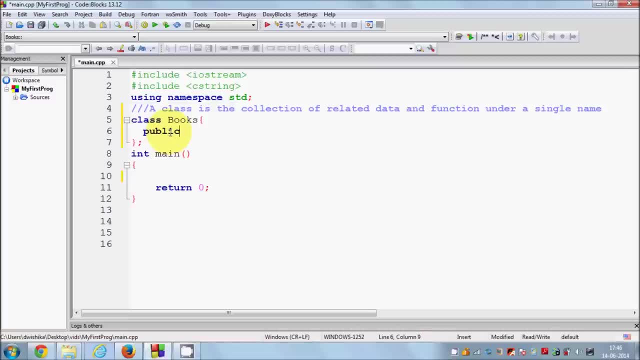 write the name public and then give this colon, Not this, but this colon, And whatever you write under this will be considered or will be treated as public members of this class. For example, I declare a variable int and I will say the book id. So I will declare: 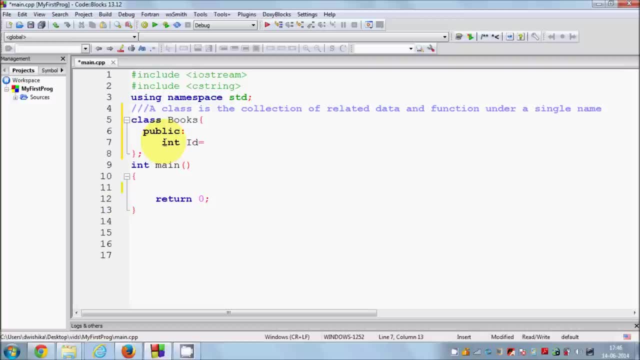 it book id And I will declare a function also inside this class to print the book id. So I will say void, print book id. And I will give this parenthesis and int And inside this I will just print the book id. So I will say cout, the book id is equal. 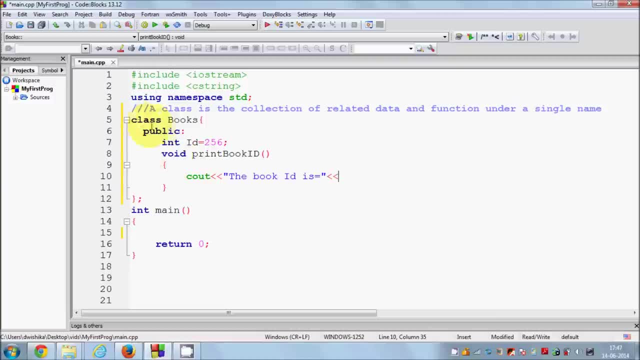 to, and then I will just copy this book id, paste it here and end line. Okay, Now I have declared a variable inside my book class and I have declared a function inside my book class. So you can declare variables and functions inside your book class or inside. 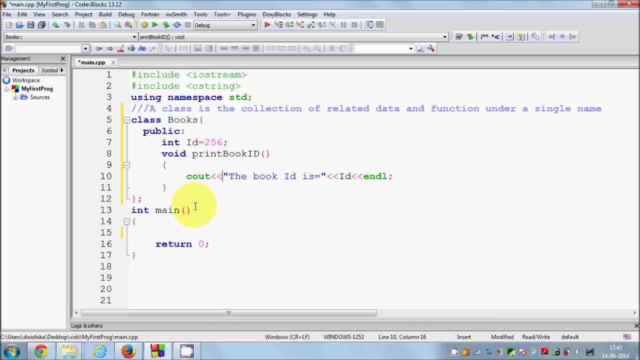 your any class Right Now. for example, you want to use these members or this function in here inside your main function. What you need to do is you need to declare an object of this class. And why do we use object? Because there can be many classes inside your program. 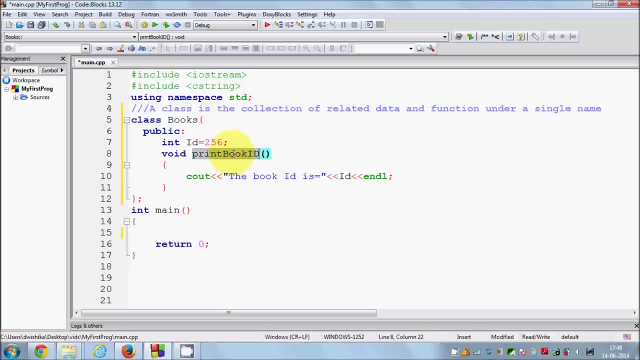 and there can be functions which have the same name. For example, the other class can also contain print book ID, The other class can also contain ID. So there can be multiple definition of these functions. And how will you know which class this function belongs to? So for this you need: 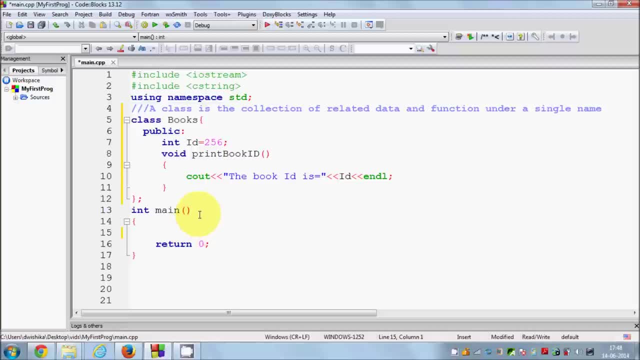 to declare object. So you know which class this function belongs to. So an object is an instance of the class. Now, to declare the object, what you need to do is you need to use the name of the class. So I will just use the name. 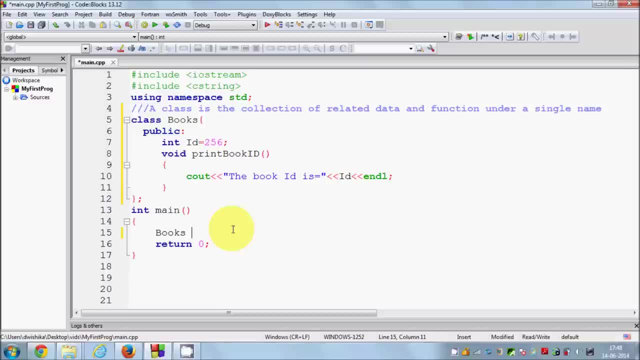 And then you need to give the variable name or object name to this. So I will give the object name. for example, book one and semicolon. So this variable or this is called the object of the class And we will, we are going to access the functions inside this book class or the class. 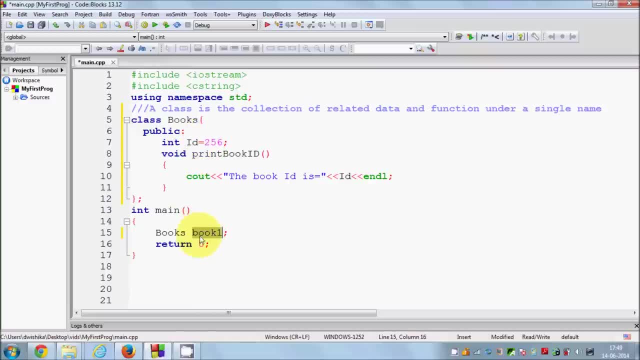 Or variable inside this book class using this object. Okay, So how we can use this function print book ID using this book one object, just write book one And we use this dot separator in order to access this function. So I will use this print book function and just semicolon, And then now I 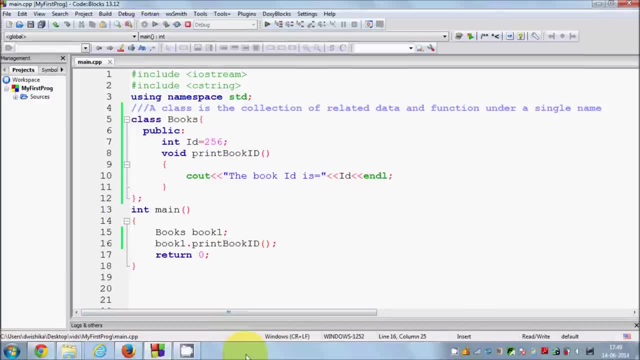 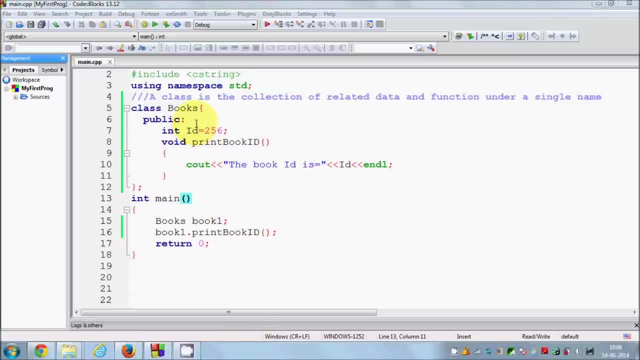 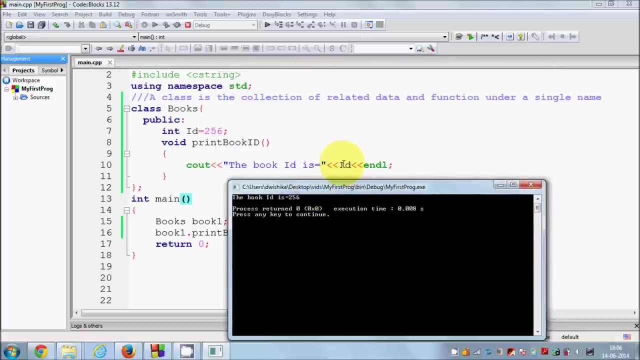 can just Compile my program And hopefully it will not give me any errors. So my program is built now And now I can run my program. So I will run my program and you can see the book ID is and whatever the ID of the book, Right. So in this way you can declare objects of a class and you can 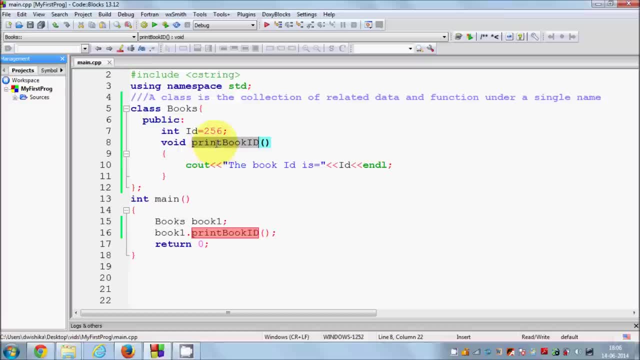 access the member of the class. These are called member function and this is called a member variable. you can directly access this variable by, for example: you want to access this variable because this is a public public variable. we have declared this in public access member variable, so we can just write it here. 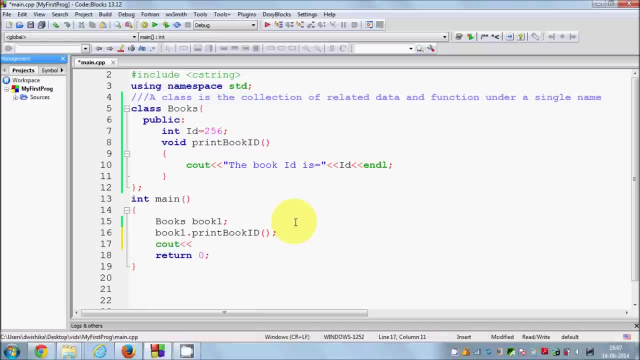 cout book 1 dot ID. okay, and this will print you the book ID, which is 256, right, so you can access this variable also, because this is a public member of this class. right, and now I will build my program and run it and you can see it.